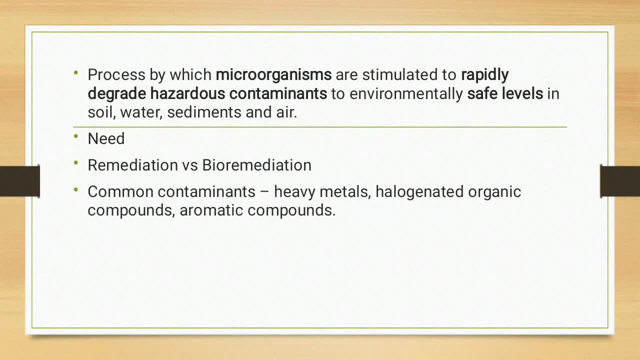 up or the pollutant is removed from there. the contaminant is removed from there, then we call it as bioremediation, and usually the microorganisms use these contaminants as an energy source or as a carbon source. In some cases they may even use it as an electron source, but that is rare. Usually, 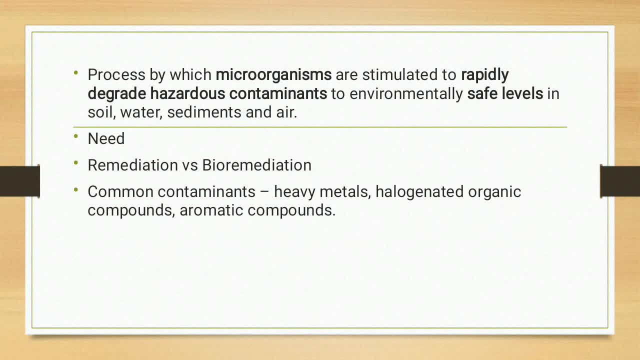 the organisms use the contaminants as an energy source or as a source of carbon. Now, why have? why did we have the need for this bioremediation? So we know that industries have increased so in multiple fold and due to public negligence it has contaminated the resources. So if we use conventional techniques to clean up that is called as the bioremediation. we have to have the standard techniques and the conventional techniques to clean up the bioremediation. So we need to have the standard techniques to clean up the bioremediation. So we need to. 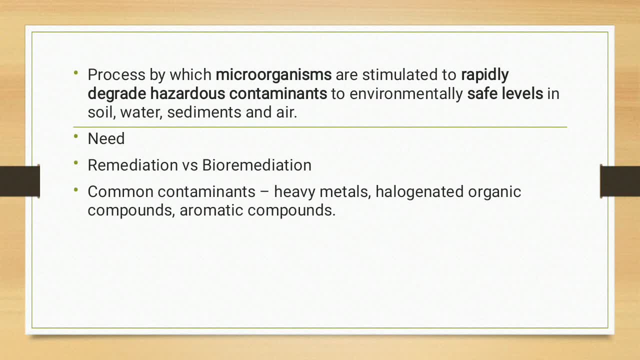 remediation. if we use conventional techniques to clean up, the first techniques were to dig up the contaminated soil, or to dig up or to take the water which is contaminated, remove it from its place and put it or transfer it into another landfill, or cap it. if it is a water body, cap it. 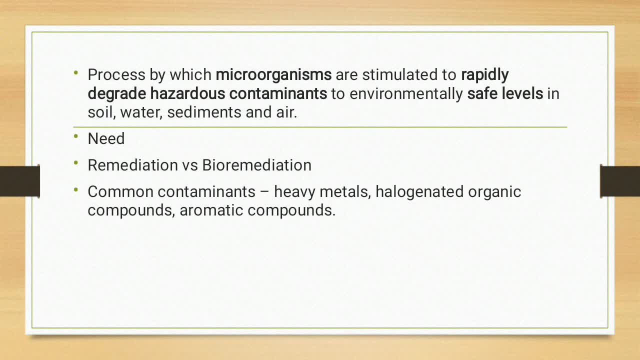 or cover it and contain the site or cover up the site. don't use it. this was the initial method of clearing contaminants, but we very well know that this is only a movement or transfer of the contaminants elsewhere. we are not actually cleaning it, we are only shifting it from one. 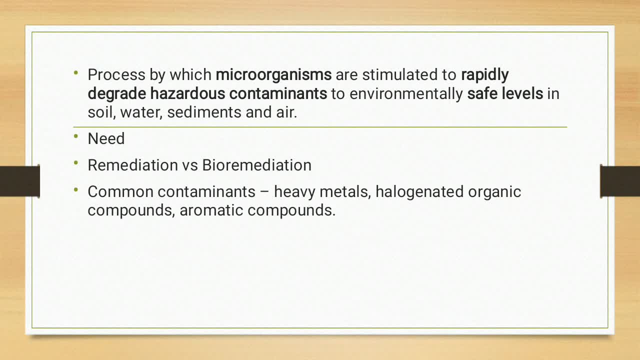 place and moving it to another place. also, when we are excavating or when we are digging up the soil, when we are handling that soil or water during the transportation, during every one of these processes there is risk. also now due to the extensive population explosion we don't have 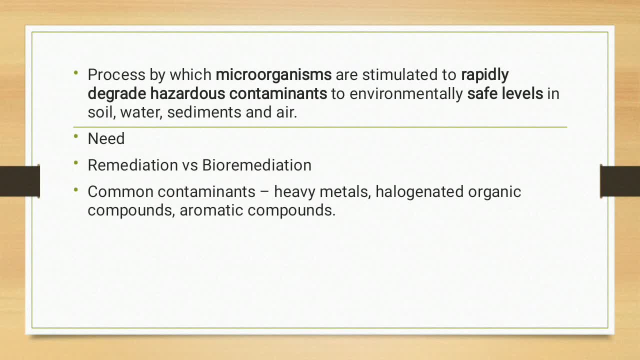 any new areas to dump it. so this led to the actual remediation. now remediation initially was being done. even now many places they do remediation chemically by using dechlorination or dehalogenation, if it for chemical decomposition or incineration, that is, burning or UV oxidation, but all of these are one. 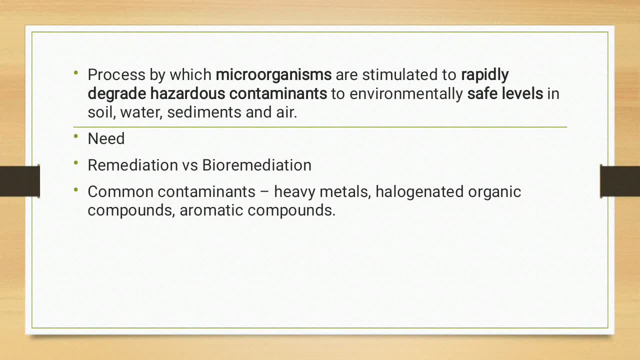 extensive in cost or they are expensive. and secondly, they cause more pollution. if you burn something, if you incinerate something at very high temperatures, it will lead to soot, because these are organic contaminants. it produces soot which enters our atmosphere and eventually causes more. 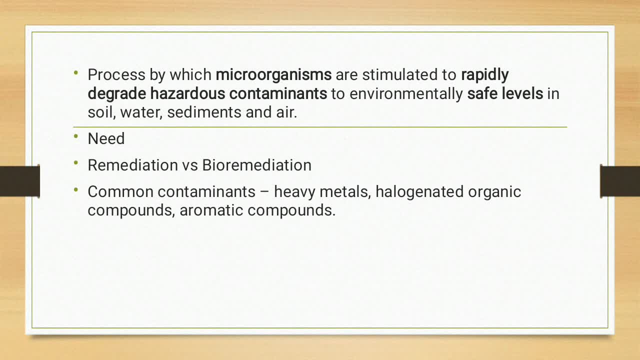 pollution. so we are shifting the contaminants from one area but adding on to pollution of another biosphere. this is when the bioremediation was introduced and you know it was mooted to be the best option because it is relatively low cost, it is not using much of technology and though it 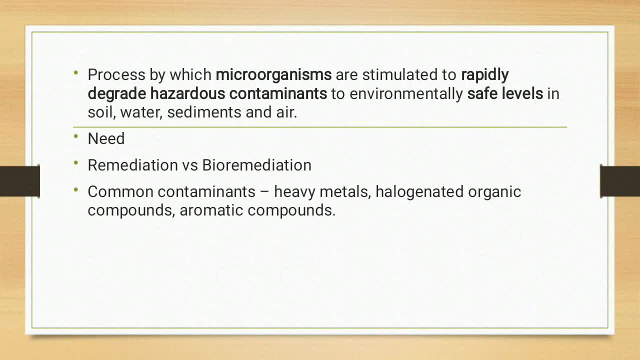 has not been extensively used in all the places. it is being applied in many parts of the world. so the common contaminants for which we found that bioremediation can be applicable. now it cannot be used for all the contaminants we haven't found ways to use. as of now we know that this useful against contaminants like heavy metals. 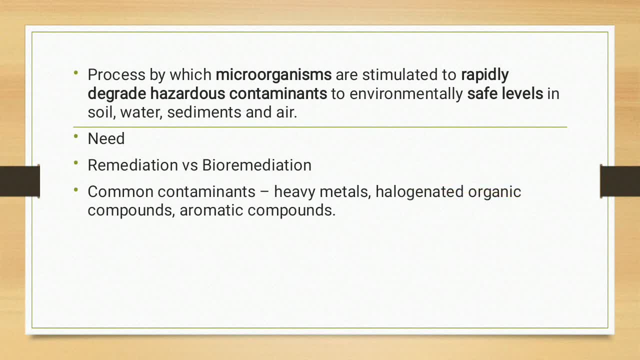 against halogenated organic compounds. this includes chloromethane, trichloromethane, trichloroethane, all the chlorinated alkenes, chlorinated alkenes- all of these come under halogenated organic compounds, and aromatic compounds such as chlorobenzene, again halogenated. 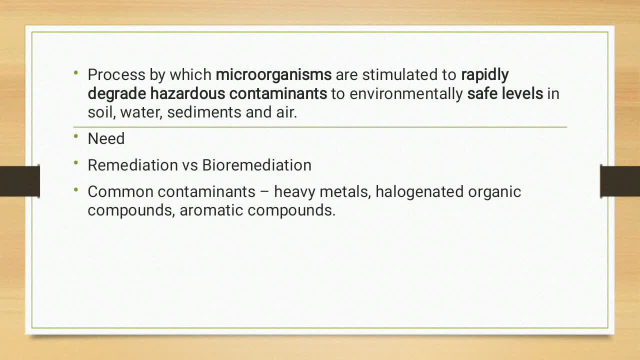 organic aromatic compounds are used for the use of chloromethane and trichloroethane and other compounds like chlorobenzene, dichlorobenzene or chlorinated phenols. all of these components which I am talking about are used in pesticides, in herbicides, in detergents, so they are ample. 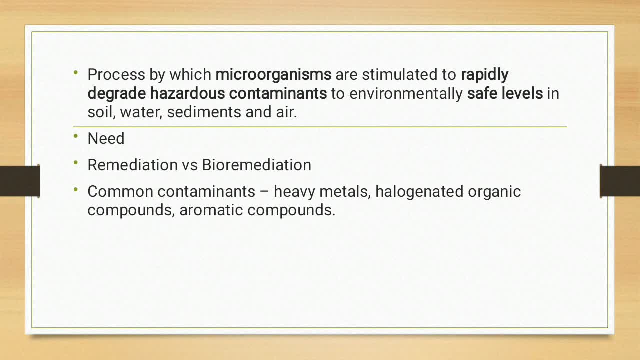 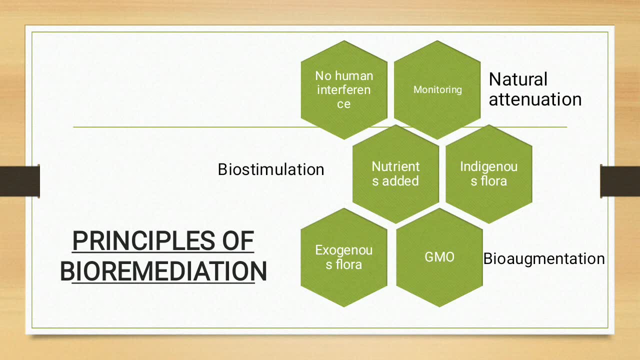 in the environment and it has been found that bioremediation is a tool which can be used to clear up these contaminants. so, coming to the principles of bioremediation now, there are three principles: natural attenuation, biostimulation and bioaugmentation. now, whatever I have listed, 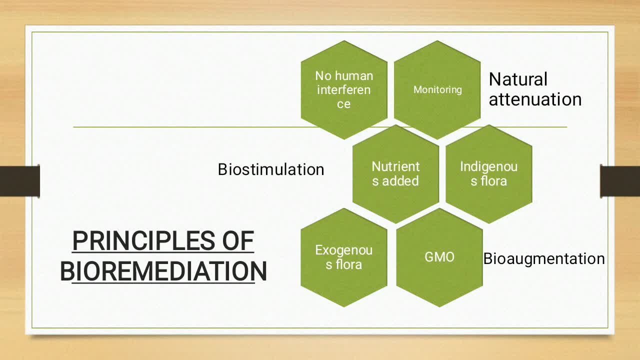 here are the principles for microbial bioremediation. we also have one more category of bioremediation, that is phytoremediation. phytoremediation is where we use plants to remove the contaminants, so the plants are able to draw the contaminants into their structures and they hold on to them. 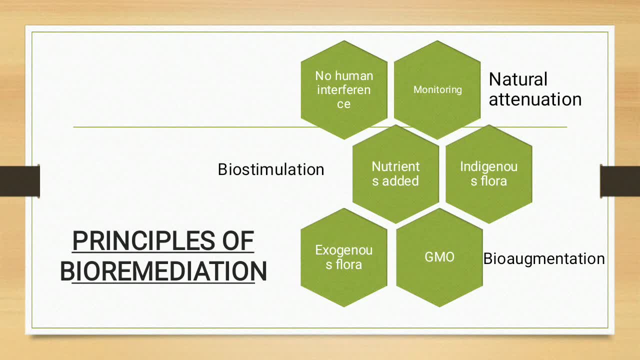 thus effectively removing them from that particular soil or water, some of the common plants being Indian mustard or water hyacinth, willow plant, poplar tree, sunflower, etc. there are many plants which are known to show phytoremediation, that is, they absorb these heavy metals or organic contaminants and hence it is removed from. 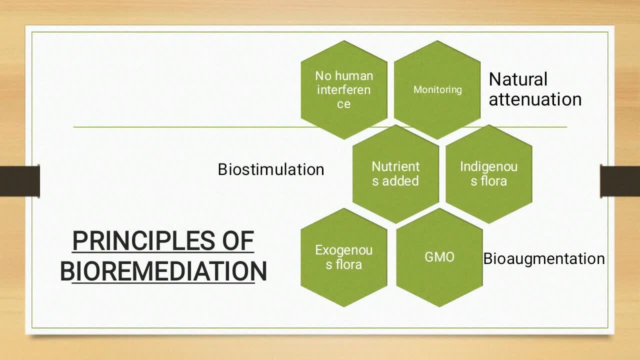 that particular and environment or from that particular soil. but what I have shown here and what we are more dealing with in this paper of environment and microbiology is the principles of microbial bioremediation, where you use microorganisms. so microorganisms produce several enzymes as part of their metabolism. they also break down complex organic and inorganic. 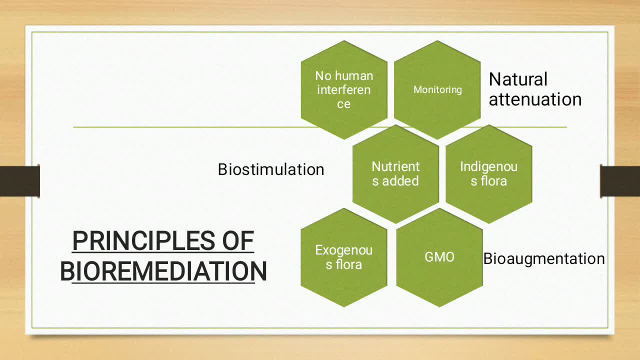 compounds. At times they are not bioremediated. Sometimes microorganisms could be naturally present at a particular site. Those are called as indigenous flora, organisms which are native flora, which are already present at a site, or the people who are doing bioremediation can add. these organisms can bring them from elsewhere. 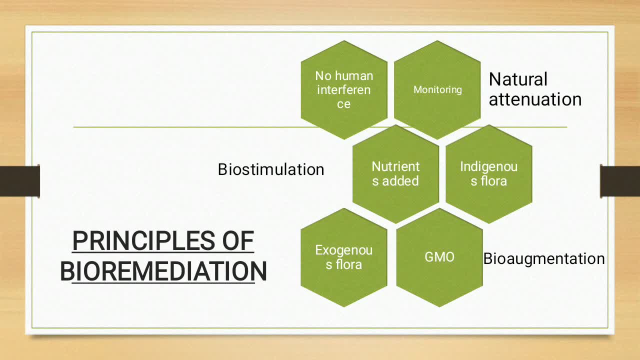 and add it to the contaminated site. So, based on all this, there are three modes or three principles of bioremediation: natural attenuation, biostimulation and bioaugmentation. Now, natural attenuation is a type of bioremediation which occurs without human interference, So we 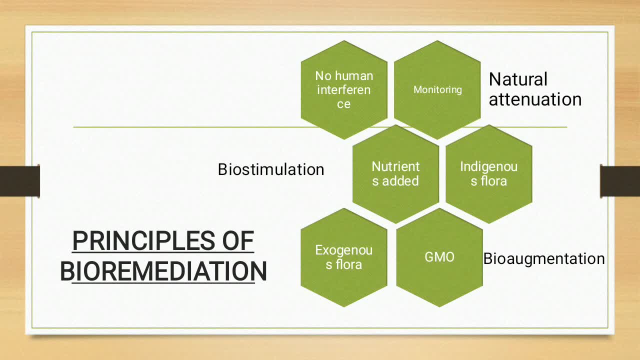 do not add anything there. we do not add any flora, we do not add any microorganism, we are only going to monitor, and thus it relies on the indigenous flora Only. monitoring is the human part of it. we do not add any other organism and we are relying on the indigenous 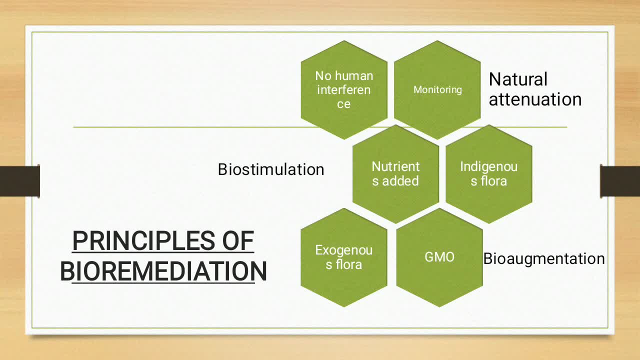 organism. So this is the type of bioremediation which occurs without human interference. So on the native flora to do their job of cleaning up. that is called as natural attenuation. Biostimulation is where we again use the indigenous flora. we are not adding microorganisms. 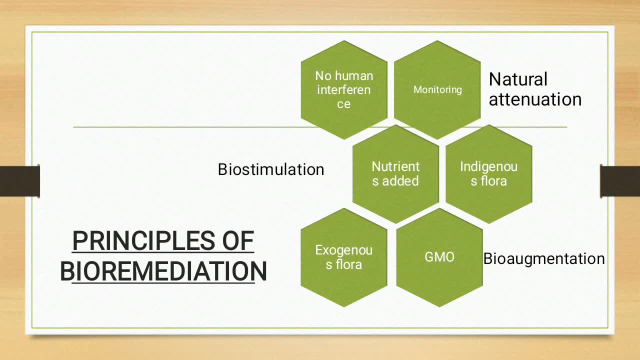 but this involves addition of nutrients which can catalyze the natural attenuation. or we are adding nutrients which are helping the indigenous flora to degrade the particular contaminant faster. So they are catalyzing, they are increasing the pace at which natural attenuation occurs. But here also, 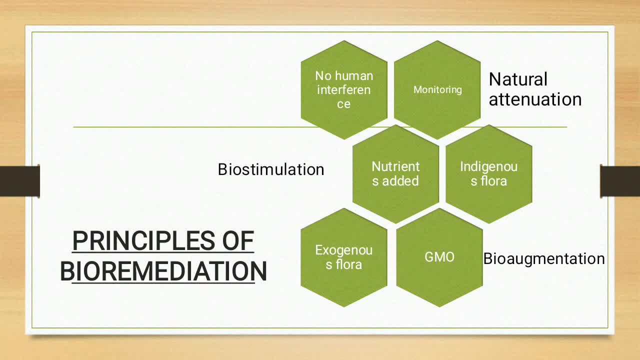 we are going to use the indigenous flora itself. The third one is bioaugmentation. Now, here there is involvement of exogenous flora or organisms which are brought in from outside. they are not native to that particular environment, They are brought in from outside. 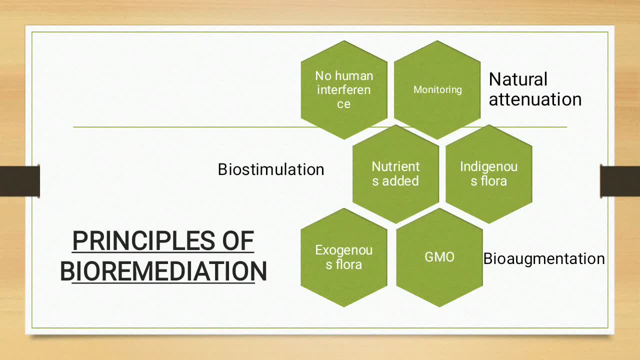 because they are able to or they are capable of destroying this particular contaminant. So these are usually genetically modified. So we would have worked in the lab to create an organism that can break down the contaminant. You bring it and add it to this contaminated site so that it can do its job well. That is called as bioaugmentation. 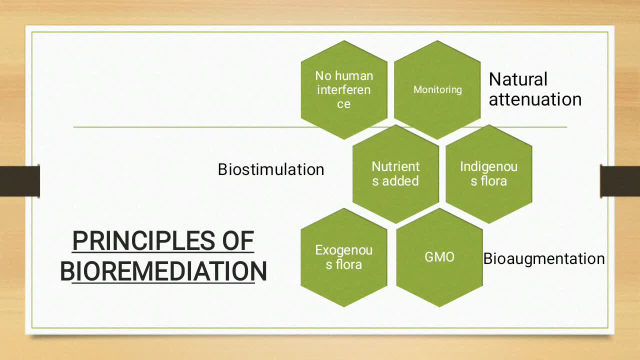 So whichever type of principle we use, whether it is natural attenuation, biostimulation or bioaugmentation, it again varies on different factors, For example the temperature or the moisture or the presence of oxygen. Some organisms don't want oxygen, they are anaerobic. 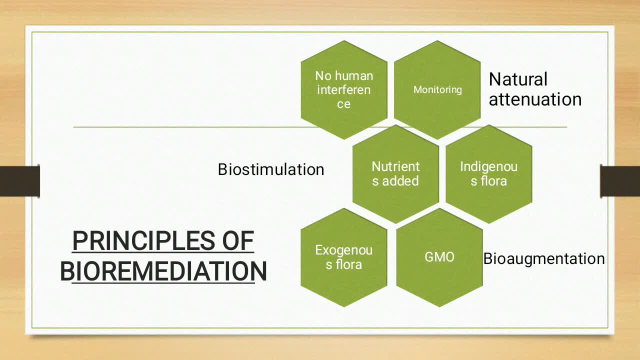 So in that case we will have to provide anaerobes. In some cases they are anaerobic, But we are going to keep them in the lab to continue doing the work. So in that case we will have to provide anaerobes. 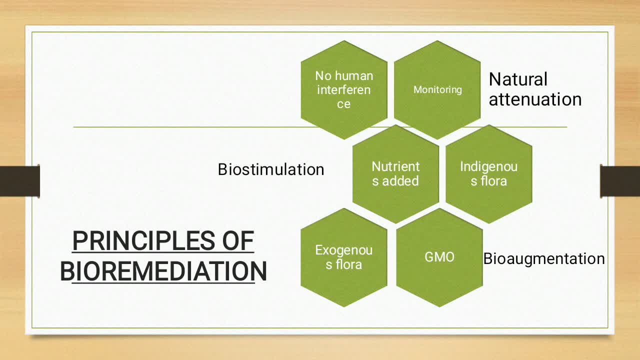 In some cases, they need a small percentage of oxygen. So, based on all these electron acceptors that are available in the environment, based on the pH of the soil or water, all of these are factors that can determine effective bioremediation. 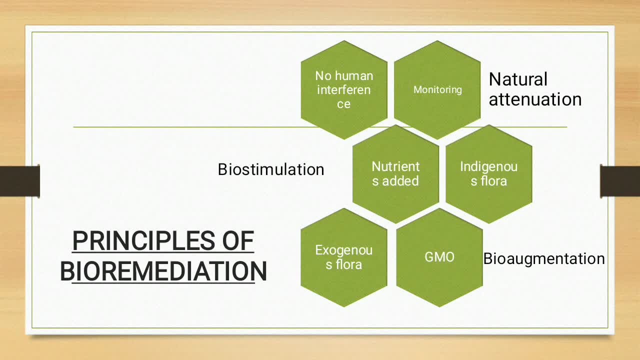 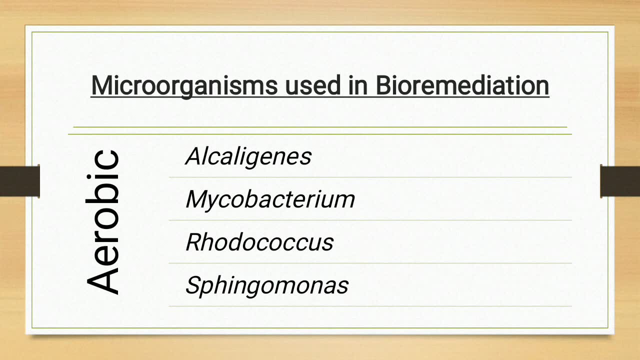 So, based on these three principles, we have several organisms that do their work beautifully. So, amongst the organisms, the first group of organisms are aerobic. This includes many examples. I have only listed out a few over here. It includes organisms like pseudomonas, very good biodegraders, alkyl genes, sphingomonas. 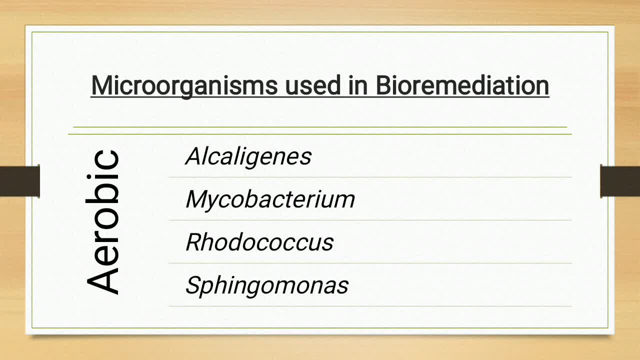 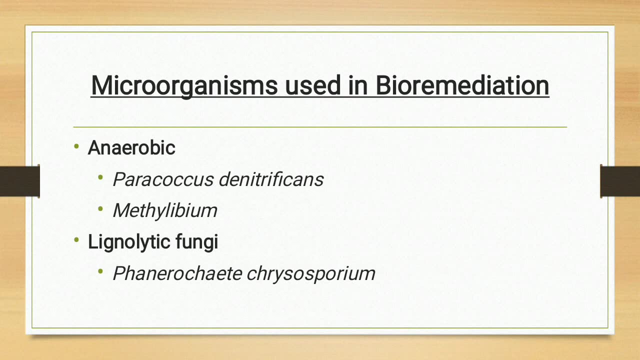 rhodococcus mycobacterium. all of these are known to degrade pesticides, hydrocarbons like aliphatic and aromatic compounds, So these are organisms that are aerobic and that are used in bioremediation. Then we have anaerobic organisms like paracoccus, denitrificans and methyllibium. 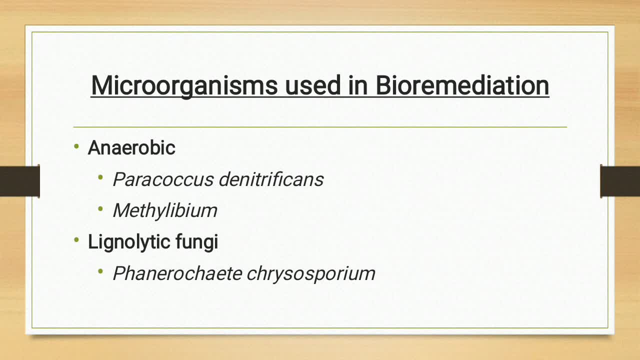 It is known that methyllibium is having enzymes that are capable of degrading polychlorinated biphenyls, or PCBs, and even chloroform or trichloroethylene compounds that are difficult to be degraded naturally. These organisms are known to have systems or metabolism to degrade these particular. 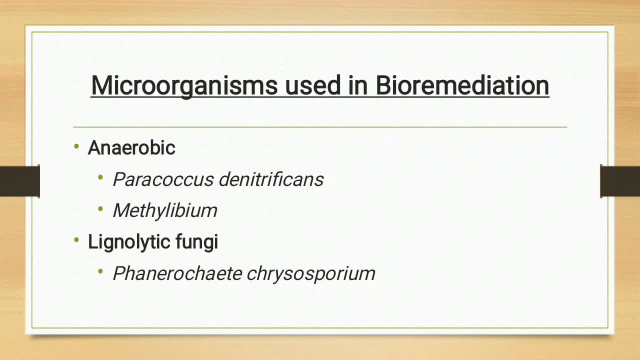 compounds, So anaerobic organisms mainly are paracoccus, denitrificans and methyllibium. Then we have lignolytic fungi like Phenerochete chrysosporium, Which is also known to show biodegradation extensively. 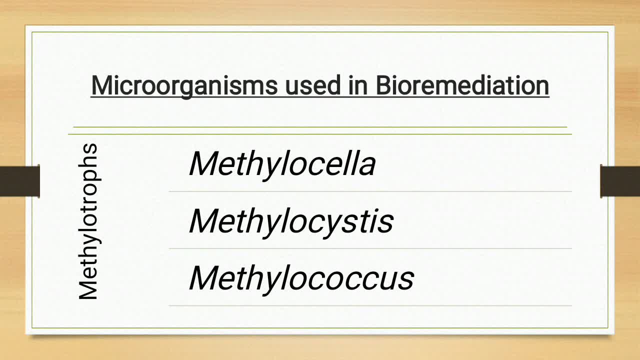 And we have methylotrophs. Now, methylotrophs are organisms. I have already told you about these. These are organisms which utilize methane as a carbon source and convert it into carbon dioxide. So amongst methylotrophs, we have organisms like methylosella, methylococcus and methylocystis. 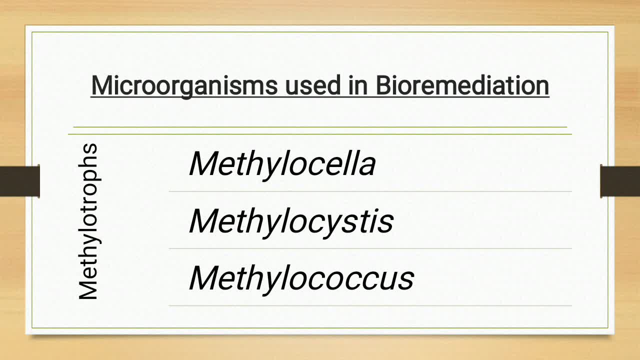 which have the enzyme methane monooxygenase. So all the methylotrophs, All the methylotrophs have methane monooxygenase And this enzyme, apart from acting on methane, though its initial substrate or original substrate is methane, it is known that this enzyme can also act upon other substrates, or it has a 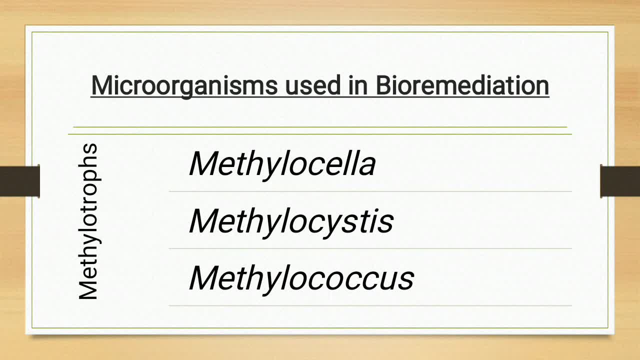 broad substrate range, like it can act upon aliphatic compounds, chlorinated aliphatic compounds, apart from methane. So methylotrophs are also an important group of organisms that can be used for bio remediation. So that means We have 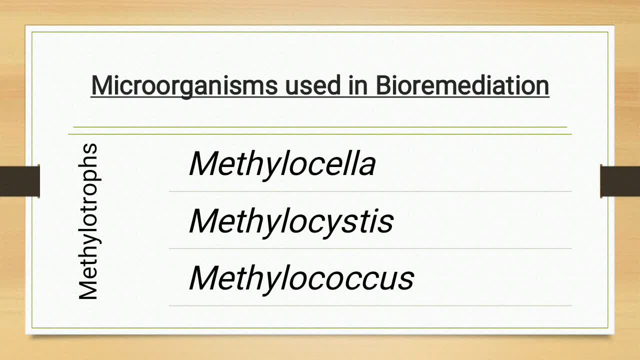 organisms, anaerobic organisms, lignolytic fungi like phenerokeet, and we have methylotrophs. These are the four groups of organisms that are mainly used in bioremediation. Now, what we spoke about earlier, that about natural attenuation, biostimulation and bioaugmentation- were the 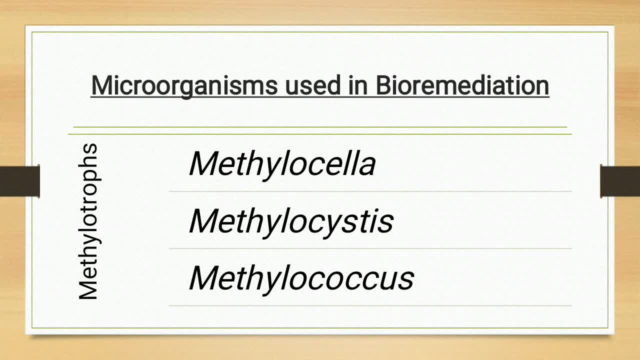 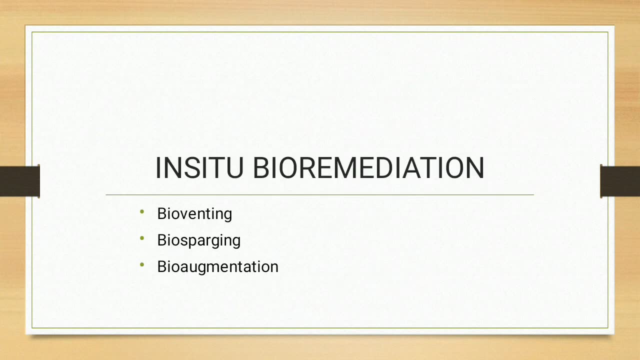 principles, But there are different strategies or different methods of showing bioremediation, which can be broadly divided into in-situ and ex-situ. In-situ methods are those where the treatment of the particular site, whether it is soil or water or sediment, in under in-situ. 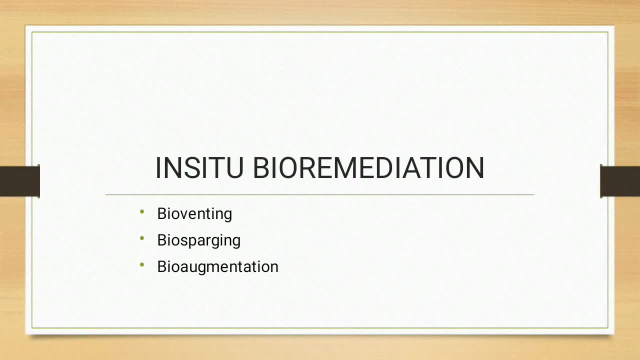 bioremediation, the treatment of the contaminated site, happens at the site. It happens wherever the contamination has occurred and minimal disturbance is caused. So we do not do excavation, take it elsewhere, dump it elsewhere, then clean up over there, then bring it back. 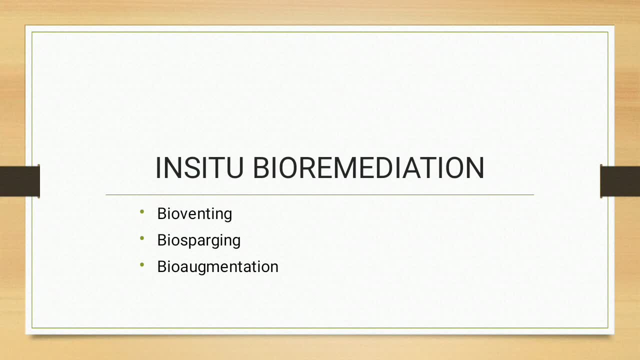 No, that does not happen. In-situ is where there is minimal disturbance to the contaminated site because treatment happens on site in-situ. Ex-situ bioremediation is wherein the contaminants are removed from the site, collected at a particular place, treated and then they are put back into. 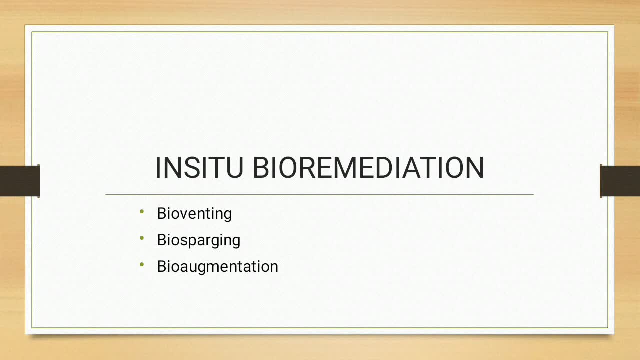 that particular site. So if it is soil it is excavated, If it is water it is pumped out. So where the treatment happens, the bioremediation occurs at a different site. it is called as ex-situ. Now, under in-situ, we again have three subtypes: bioventing: 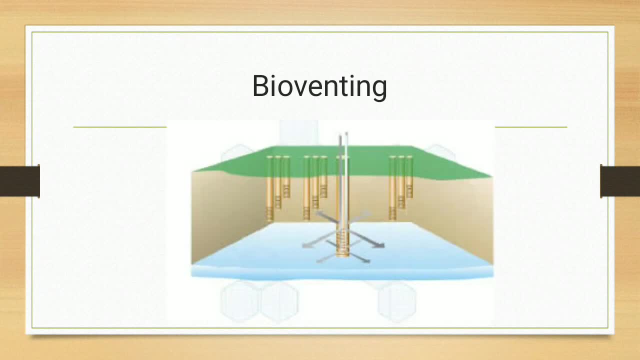 biosparging and bioaugmentation. Let us see what each one of these is. So the first type of in-situ bioremediation is bioventing. Now, bioventing is the most common method. You can see over here there are wells or channels that are dug into the contaminated soil. 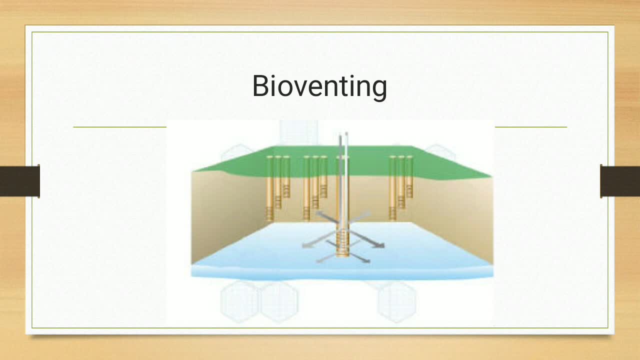 or into the contaminated part. If we want to clean groundwater, even then we have to dig into the contaminated soil. There are wells or channels or tunnels that are dug into the soil. Through these wells, air and nutrients are supplied. When these air and nutrients are supplied through the 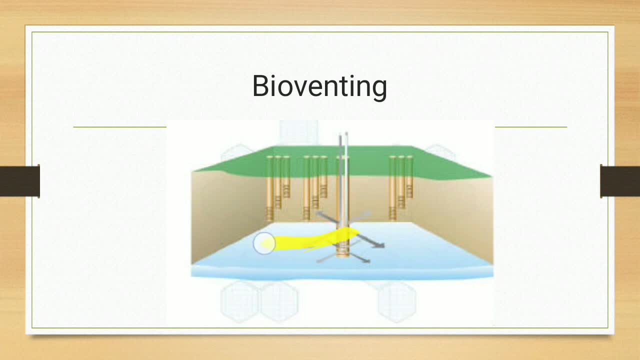 wells they are entering over here, The organisms which are already present. so we are depending on the indigenous flora. the organisms which are already present over there get stimulated, or the indigenous flora gets stimulated because we have provided fresh air and nutrients and they 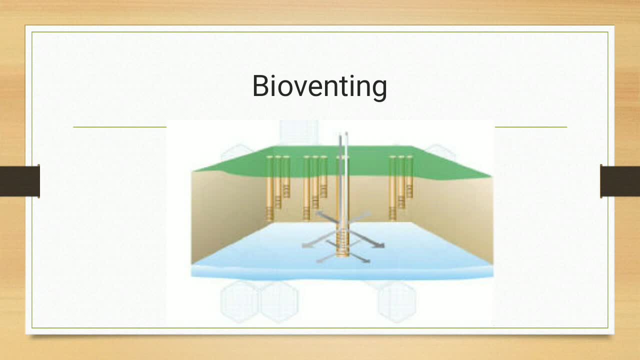 they immediately start the biodegradation, or the biodegradation occurs at a rapid rate. So bioventing is where the air flow rates are kept low, The air is pushed inside, but it is not applied with a lot of pressure and the air flow rate is very low so that there is minimum. 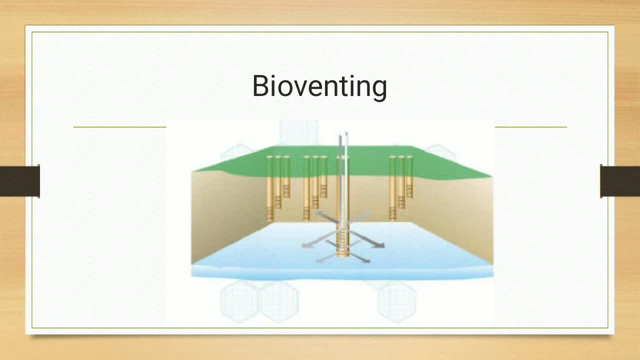 volatilization of the organic compounds. So if there are contaminants inside, if you push in air at a very high pressure, they will all start volatilizing and exiting the air. So this is a very important thing to keep in mind. So if there are contaminants inside, if you push in air at a 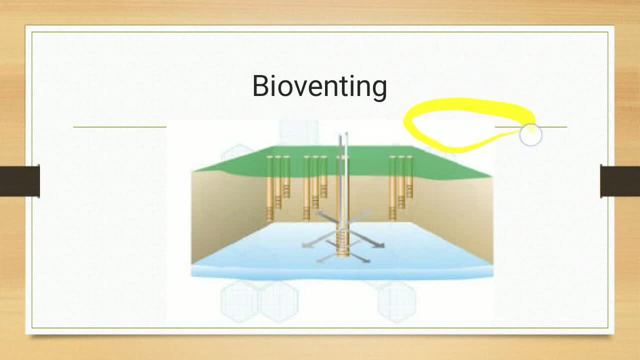 very high pressure, they will start exiting out or they will start coming out through these wells, in turn harming the people and personal working over there, or even entering into the atmosphere and causing pollution. So in bioventing, the air flow rates are maintained low so that 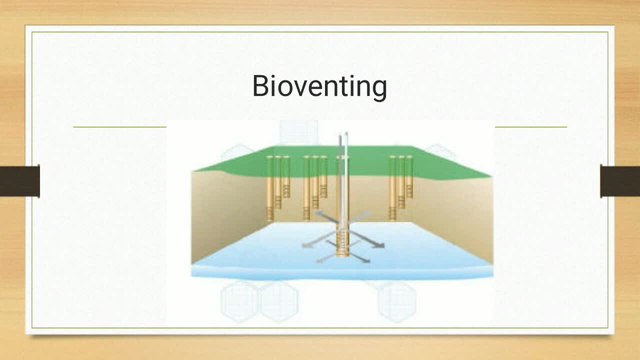 volatilization is less and the release of contaminants does not occur to the atmosphere. This is mainly used. bioventing is mainly used wherein the contamination is deep under the surface, So you just have to dig the wells, supply the air and nutrients through these wells and 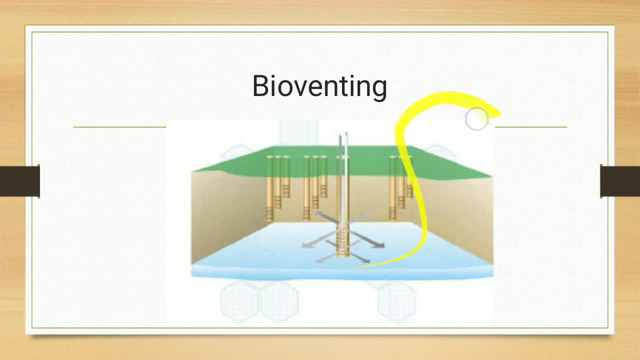 through a different set of channels. So this is a very important thing to keep in mind when you are doing bioventing. So if you have a different set of wells, we have to pump the water out or whatever needs to be pumped out or the nutrients that are supplied in through the aqua solution. 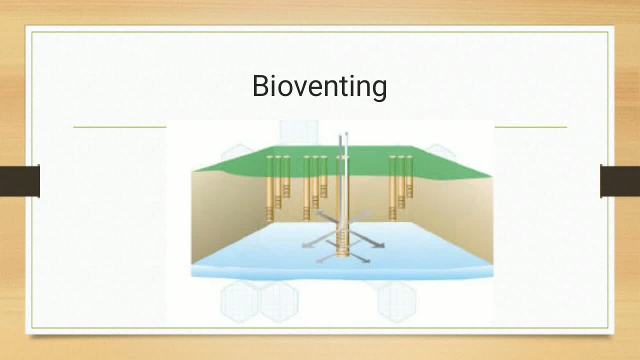 if they are supplied in through aqua solution, that will be pumped out through a different well. If these nutrients are supplied along with the air, then there is nothing to be pumped out, But there will be wells which are dug inside which can be used as an exit for the gases that. 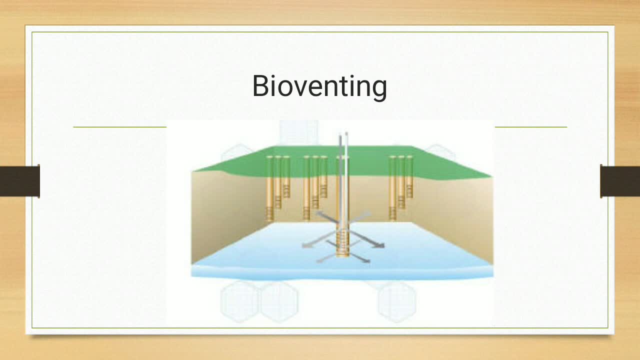 are released during the biodegradation. So this is bioventing. Main thing to remember here is: through the wells, air and nutrients are supplied, The flora is indigenous flora, no new organism is added and the airflow rates are kept low. This is called as bioventing. 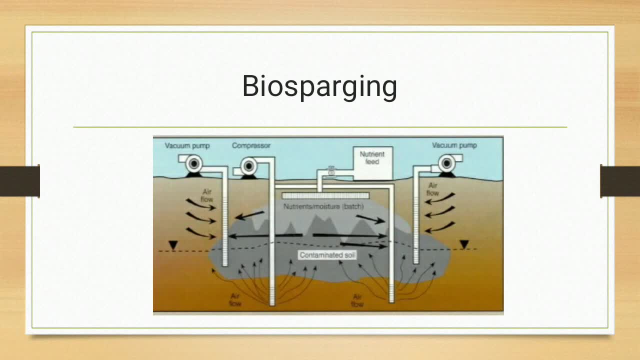 Biosparging you can see over here is also very similar, wherein you have wells that are dug inside, but the wells are attached to vacuum pumps or compressor pumps. Through these pumps again, we are injecting air under pressure, but the pressure applied here is very high, So we usually 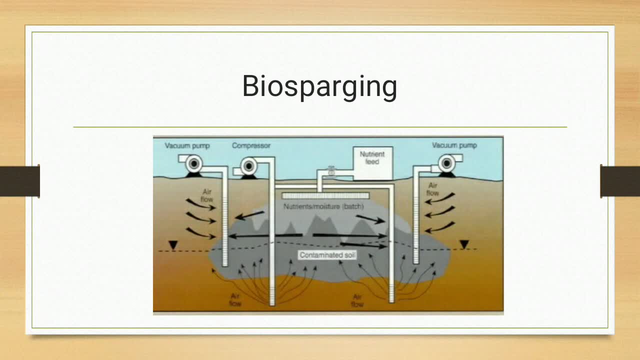 or we usually supply air and in some cases even nutrients under high pressure to increase the groundwater oxygen or to increase the oxygen present in the lower layer. So here the oxygen will increase when high pressure air is being supplied through these wells. This high pressure, that of oxygen that is supplied, will again increase the rate of biodegradation by the 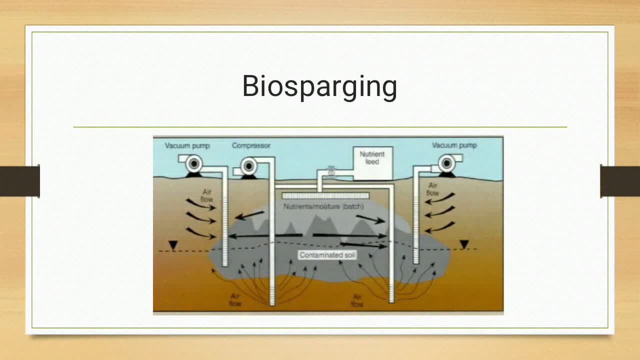 indigenous flora. So here again, we do not add organisms. we are depending on the native flora or on the indigenous flora. These organisms will degrade the components faster and we are able to clear up that particular area. In this case, what is shown is the contaminated soil, but this can. 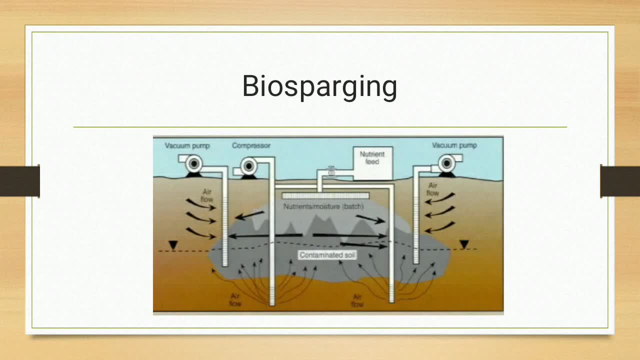 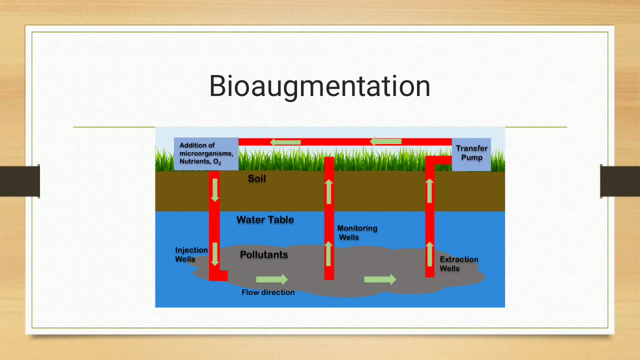 also be used for groundwater. So here we are, having air being pumped in with pressure and we are using indigenous flora. This is the what you need to remember about bio-sparging. The third one is bio-augmentation. Now, in bio-augmentation, like I told you earlier, the organisms are 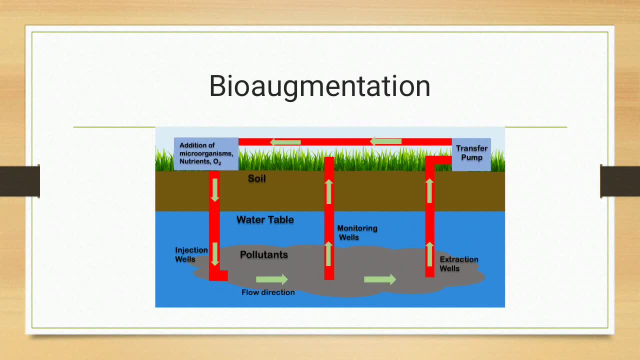 also added. So, though we have wells dug, though nutrients are being provided, we are injecting organisms as well. We are not depending on the indigenous flora. We will add flora, exogenous flora, which we know is going to perform well or which we know is going to degrade well. We add: 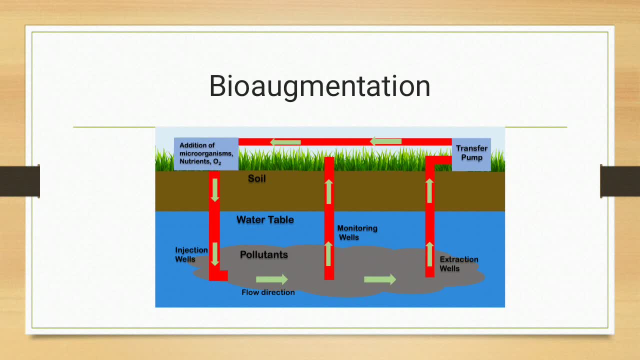 these kind of microorganisms into the pipes along with oxygen, along with the nutrients. The disadvantages could be that the particular flora we add, the organism we add, may have performed very well in the lab setting but it may not compete properly or it may not be able to compete with the indigenous flora and 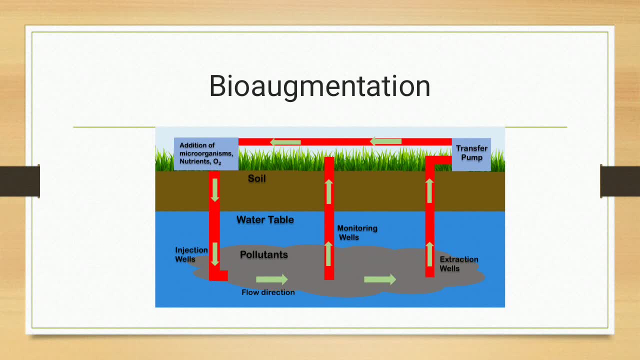 it is. there are chances that, due to the long time contamination of that particular environment, the indigenous flora might be better degraders than our particular organisms. So these are the disadvantages. but in some cases organisms are genetically engineered and they carry genes which degrade these particular organisms. It may have a negative impact on the environment. 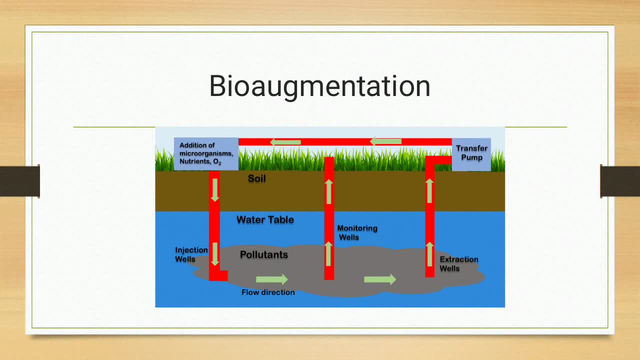 So it may really affect the environment. So here we have the undesired organisms and the particular contaminants. so these kind of organisms are added through the wells and the degradation occurs in the, at the site of the contamination. now coming to the advantages and the disadvantages of 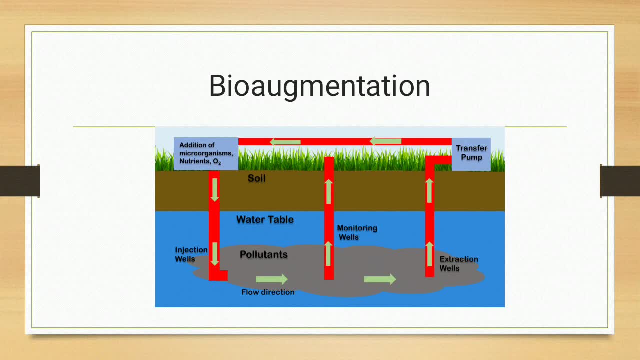 in-situ. so advantages of in-situ bioremediation is that there is minimal disruption of the contaminated site. because there is minimal disruption of the site, there is minimal risk to the personnel and the public who are working over there. also, simultaneously, we can do treatment. 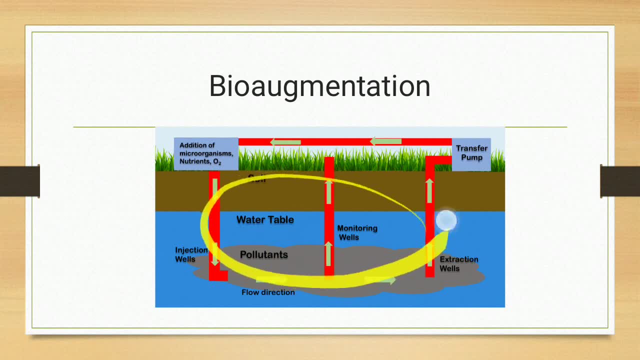 of the soil as well as the ground water. you can see over here, soil and ground water can be treated simultaneously. so that is one of the advantages of in-situ bioremediation, and it is relatively lesser in cost when compared to xc2. but the disadvantage is that this is time consuming. 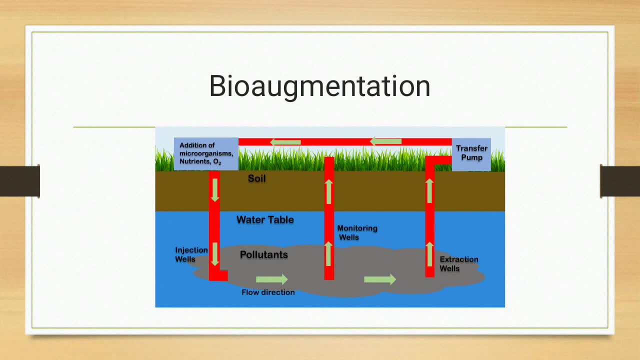 because there are a lot of factors that can occur in c2. you cannot monitor all of these factors. what are not in this environment? and you cannot monitor all of these factors in this environment? what are not in this environment? and you cannot monitor all of these factors? what are not in this? 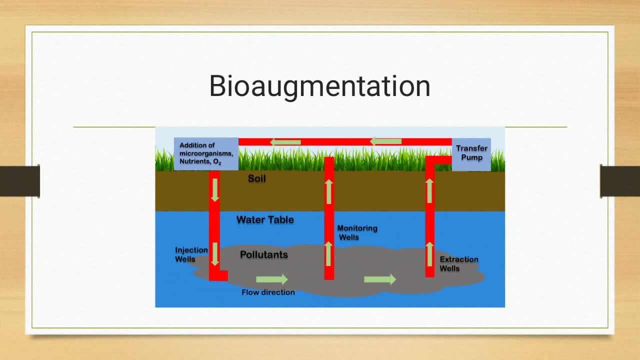 are happening inside the soil or inside the contaminated site and there is difficulty in application of the additives. so anything you need to add, you have to add through the well. there are chances that the well can be blocked. there are chances that there may be other organisms using 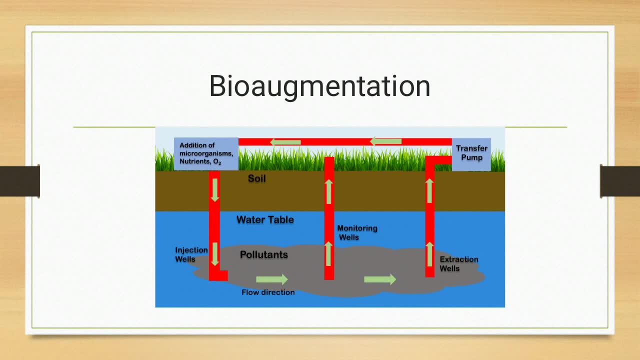 these additives that you add. so all of these issues can occur with in-situ bioremediation, but there are some advantages as well. to get over these disadvantages or to make sure that these disadvantages of time and difficulty in monitoring and application of additives is not. 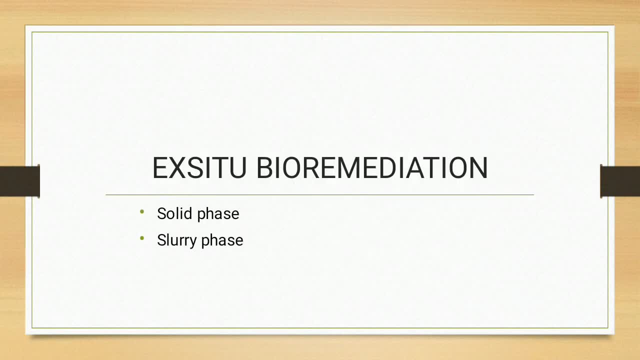 there. we have several methods of ex-situ bioremediation. so i told you earlier, ex-situ bioremediation is wherein the particular contaminated area is taken out to a different place, treated and then put back now. ex-situ bioremediation can be done either in solid phase, 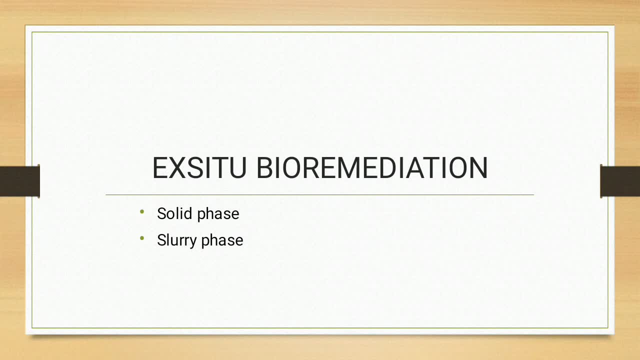 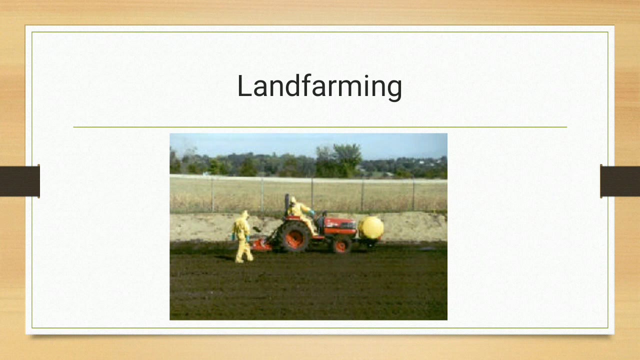 or in slurry phase. solid phase is example. examples are land farming, composting and biopiles, whereas slurry phase example is bioreactors. we'll study one by one, so the first one is land farming. this is a type of solid phase ex-situ bioremediation. 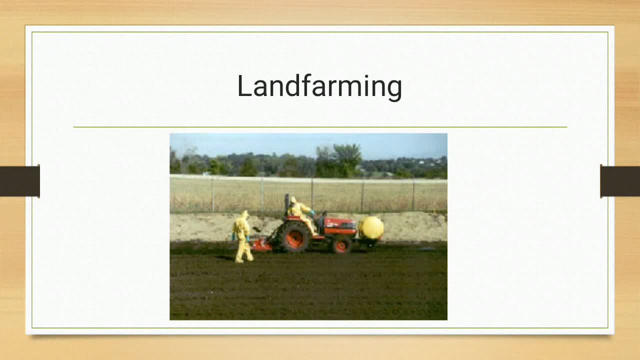 when we say ex-situ, we have taken out the particular site or we have taken out the contaminants from that site and we are treating it elsewhere, so the contaminated soil is excavated. now this is done for soil or sediments, so the contaminated soil or sediment is excavated. 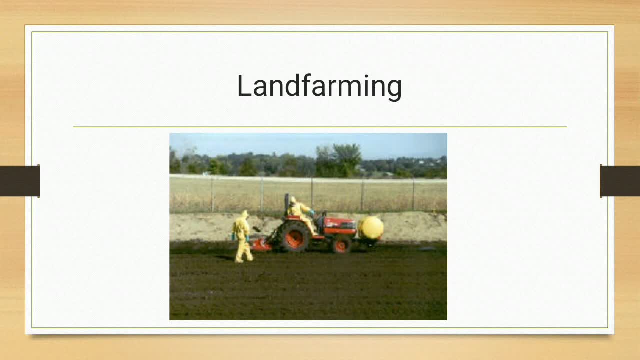 and it is spread over a bed, or it is spread over a large area and periodically this area is tilled or it is mixed till the pollutants get degraded. so here we don't add any organisms, we are basing on the indigenous flora to aerobically degrade the contaminants. but why do we not let the indigenous 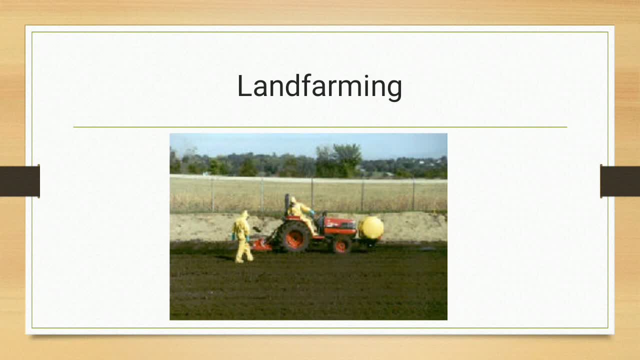 flora do it at the site, because when we take it elsewhere, monitoring is easy. so we keep tilling it. Every time we mix it, more and more oxygen is provided so that the organisms can aerobically degrade the contaminants. The second one is composting. 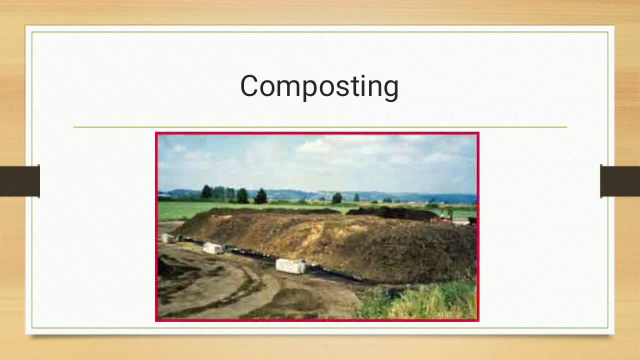 So composting is wherein the contaminated soil is excavated and it is mixed with some organic material like manure or agricultural waste, and then the degradation is allowed to happen. So it is similar to land farming, but here we don't let only the indigenous flora do the work. 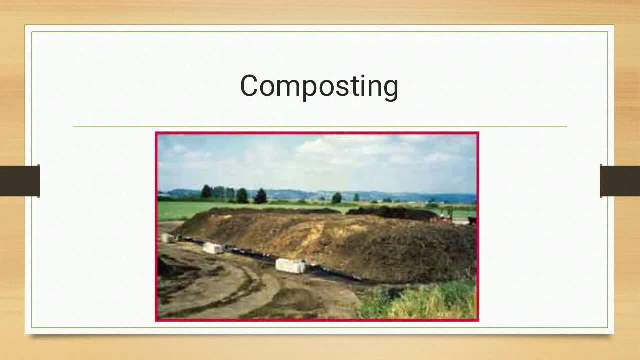 Along with the contaminated soil which has been excavated, we add some organic materials like manure. These contaminants, what are present in that particular area or in that particular soil, even if they are resistant to degradation, they can get converted to compost. So, even though they are resistant to fully or complete degradation, it has been seen that the hydrocarbons, like aliphatic hydrocarbons or aromatic hydrocarbons, do get converted into compost. 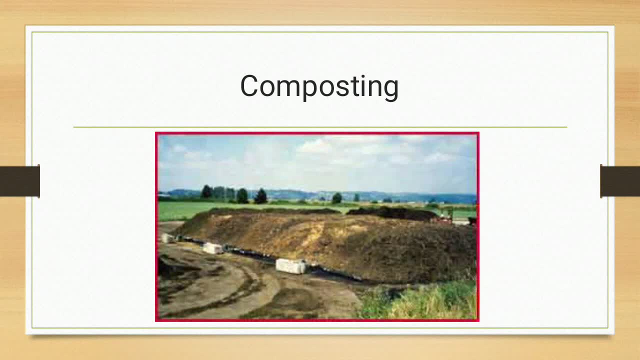 Which can be utilized for plants or which can be used for growth of the plants on an agricultural field or elsewhere. So composting is similar to land farming, but instead of just taking out the soil and mixing it, we are adding some compost to it which has organic material, which has composting flora in that. 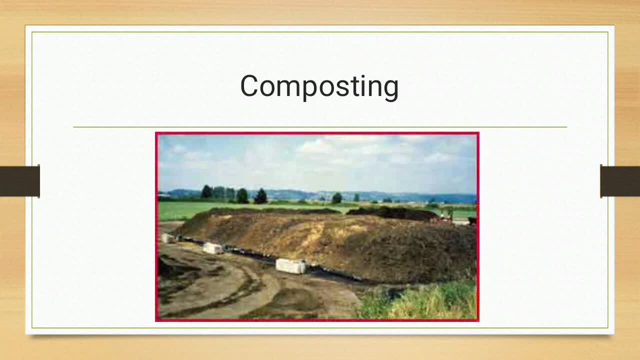 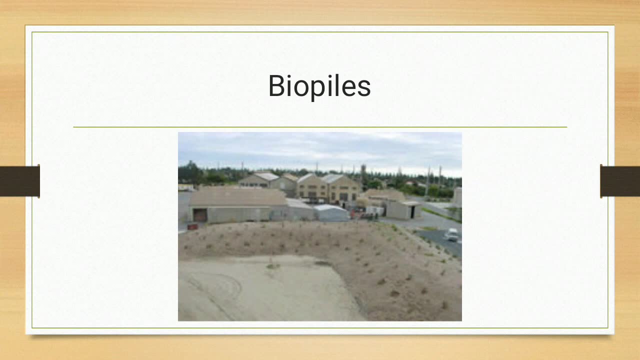 So the flora will degrade the contaminants as well to form compost. The next one is biopile. This is also coming under. This is a hybrid of the first two methods, that is, a hybrid of land farming and composting. So this is mainly used for surface contamination, not for very deep contamination, wherein we again excavate the soil and transfer it onto a new surface. 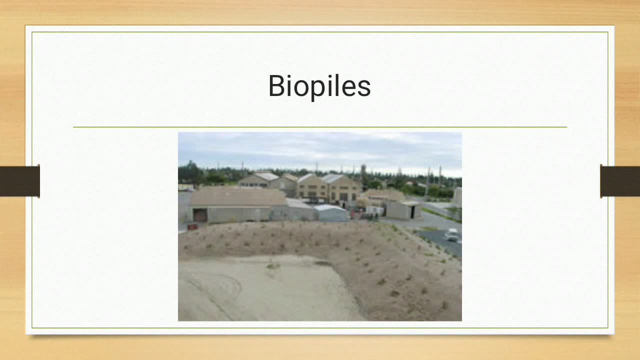 We keep tilling it. There is compost that is added, or there is manure that is added, We keep mixing it. The difference here is that it is a refined form of compost. It is a refined form of land farming because here, whatever losses are occurring by the leaching, or whatever water is getting leached out, that is also controlled, and volatilization, whatever is happening, is also controlled. 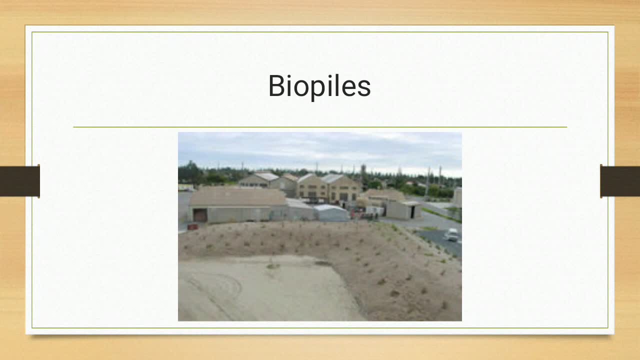 So it is only a refined form of land farming wherein volatilization and bio leaching- or leaching not bio leaching- wherever the leaching of all the components occurs. both are being controlled. That is called as biopiles. 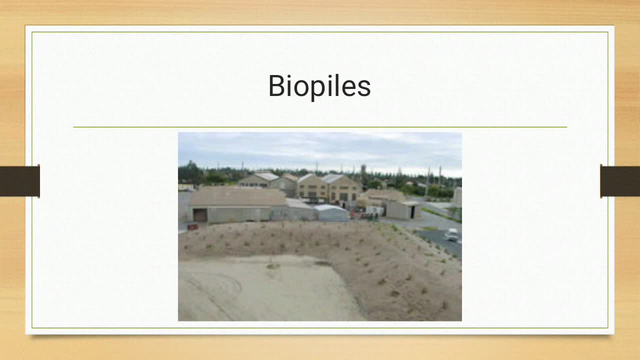 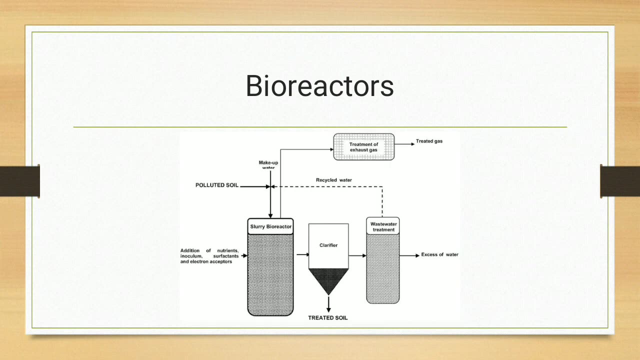 So it is similar to that of land farming. So it is similar to that of farming and composting, just that the monitoring is better. The fourth type of XC to bioremediation is bioreactors. These are also called as slurry reactors. 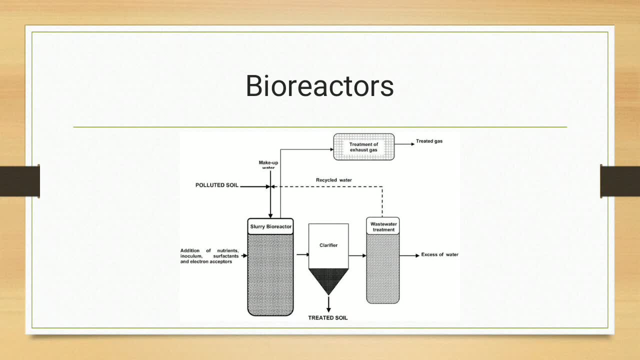 So this is the slurry phase. It is called as slurry because there is mixing of water, solid and air. Everything is getting mixed. So the solid- soil or water, sediments, whatever needs to be cleaned- is mixed with the water and then the cleaning occurs or remediation occurs. 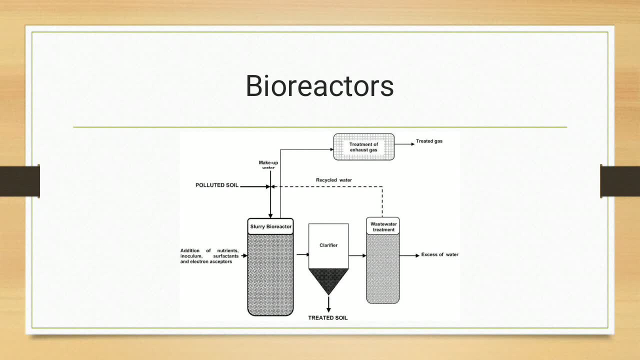 That is why this is called as bioremediation. This is called as slurry phase or slurry reactor. This can be used for solid material, cleanup of solid material, cleanup for water or air. Bioreactors can be used And in this case the rate of biodegradation is much, much higher than in in C2 or any of the other XC2 methods. 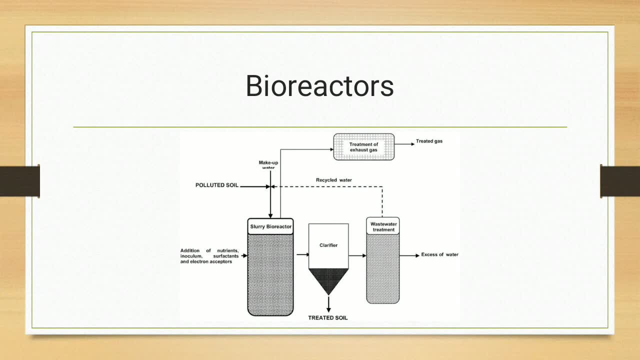 The limitation is that the cost is very high, So we need to have a separate slurry bioreactor built in which all these processes can happen, due to which the cost goes up And the soil cannot be cleaned. It cannot be added directly. 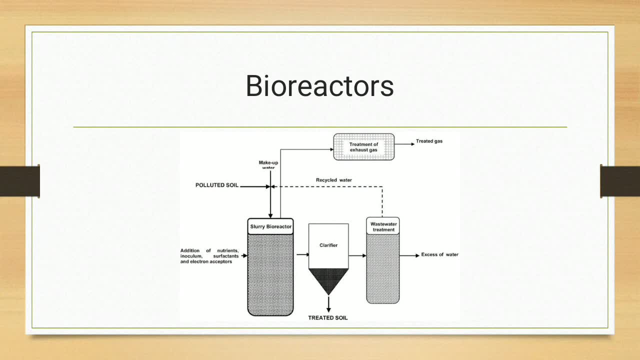 It needs pretreatment. So big rocks have to be removed, All the vegetation has to be removed, Then only it can be added into this bioreactor for the bioremediation to occur. So that pretreatment takes money And even the running of the entire system. the setup of the system takes, you know, is expensive. 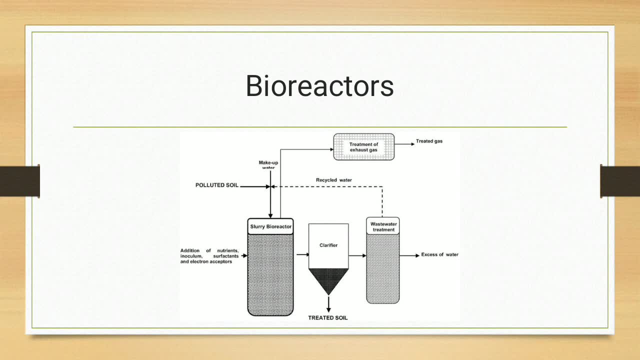 But the benefit is that it is very, very effective because we are optimizing all the parameters. I can control the temperature, the pH, I can decide when what nutrients are needed, What nutrients have to be added When I have to add water. 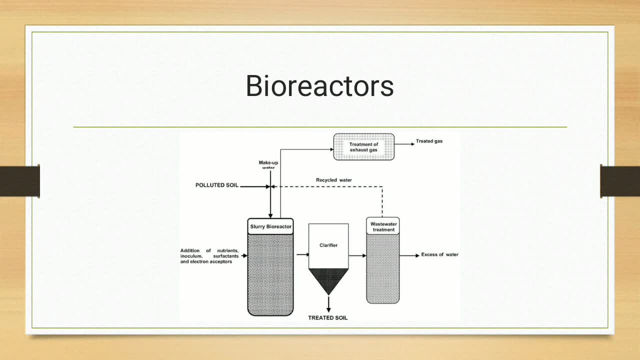 When do I have to add oxygen? Everything is very well controlled, because of which the bioremediation is very effective Under this. so examples of bioreactors are either low shear airlift reactors- I will show you the picture in the next slide. 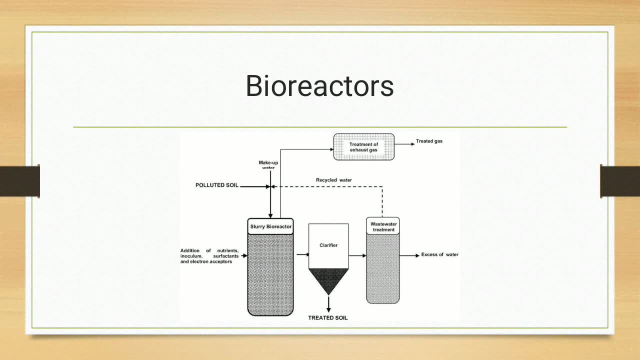 Or even aerated lagoons which are outdoor pond, like areas which are continuously aerated. They are also a type of slurry reactors, Or they are systems wherein the parameters are optimized and controlled and the bioremediation occurs in a slurry phase. 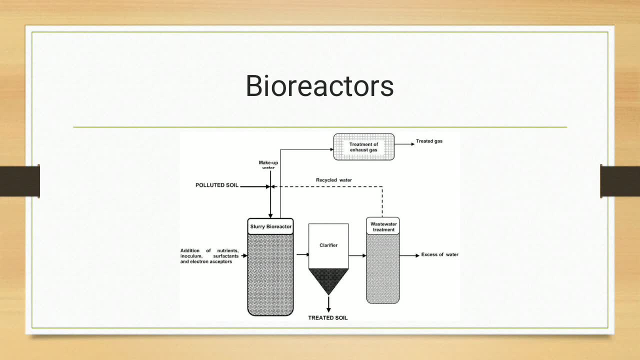 Slurry phase is where solid is being mixed with the water. So these are the different methods of bioremediation of either a solid component like soil or water, sediment or even water, Moving on to bioremediation of air. So bioremediation of air is mainly done like I told you in the previous slide. 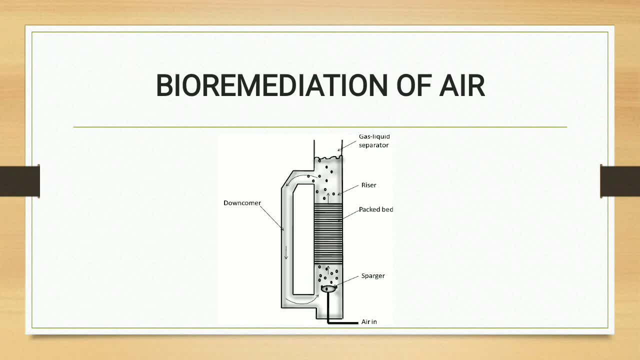 Through bioreactor. You cannot do bioremediation of air by land farming or composting or any of those methods. Bioremediation of air occurs through bioreactors And the type of bioreactor is called as airlift bioreactor. 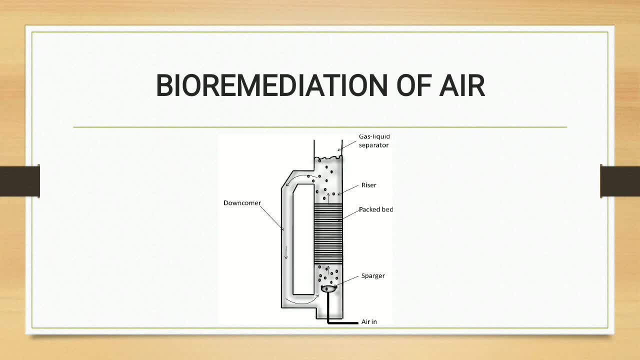 Under airlift bioreactor. it occurs by the external loop airlift bioreactor. So when you do your industrial microbiology you will see that we have internal loop and external loop airlift bioreactors. This is an example of external loop airlift bioreactor. 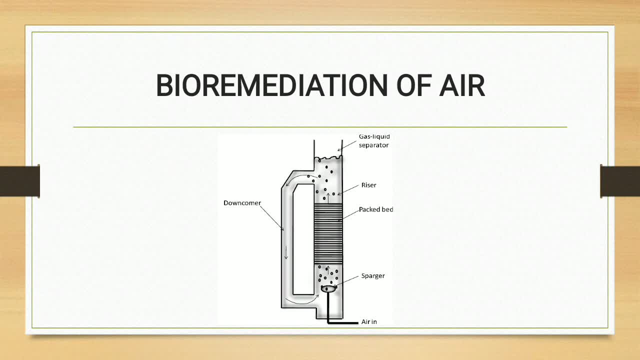 And it is seen that in this kind of a bioreactor 99.7% of contaminants are removed. So in this bioreactor it is called as external loop, because here the air keeps on circulating. If you see, here there is no separate pump to mix the air like how we have in the other bioreactors and fermenters. 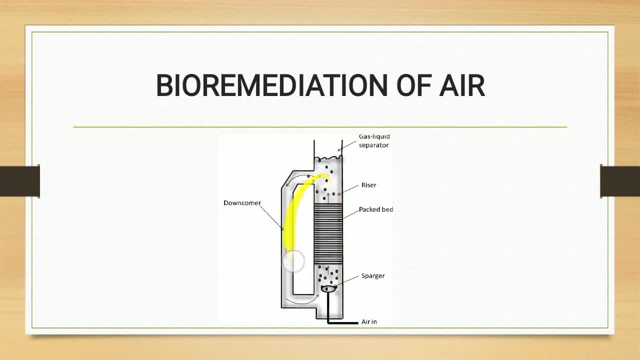 The air, as it keeps moving itself, does the mixing of the components, And the mixing happens through an external loop. that is why it is called as external loop airlift bioreactor. It has been seen that this is used for conversion of volatile organic compounds, that is, VOCs, in the air to harmless products. 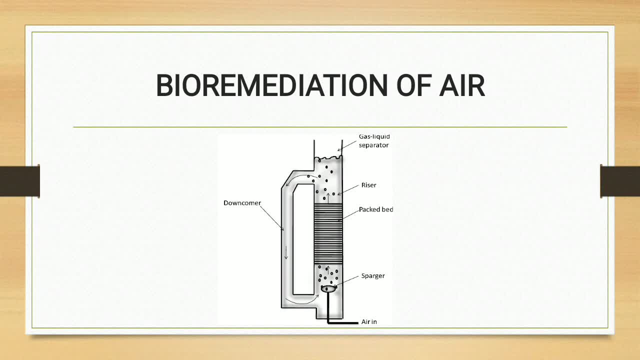 And mainly for this, algae are used and Pseudomonas putida is used. These are the organisms that are used in case of bioremediation of air. Now coming to the advantages and disadvantages of bioremediation. So bioremediation's advantages is that it is lesser in cost in comparison to chemical remediation. 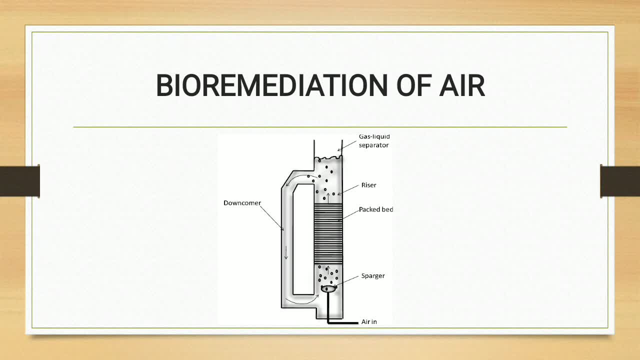 It is, it will produce residues that are harmless, like cell biomass or carbon dioxide or water, which are much less harmless than the chemical residues that are produced in other methods of remediation. Also, if it is carried out on site, that is, in case of in situ, then there is no major disruption. 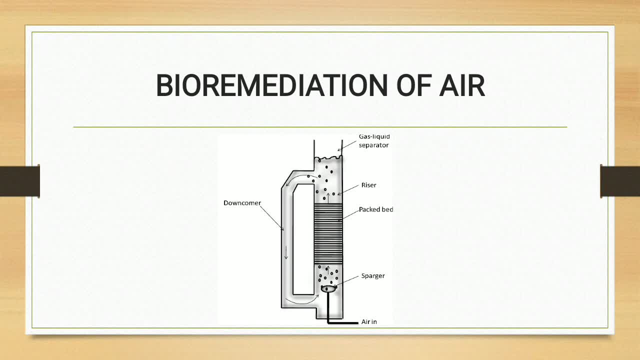 There is very less threat to the people who are working And it can be done on a variety of occasions. So bioremediation of organic and inorganic compounds. But why is then bioremediation not being applied everywhere? Because there are a few disadvantages. 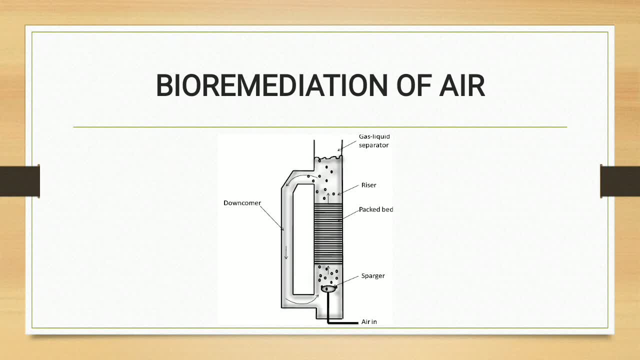 What are the disadvantages? So the main thing is the type of compound is very limited. We now know organisms of a very limited range of biodegradable compounds. Apart from that, we don't know how to degrade the other contaminants in soil or water. 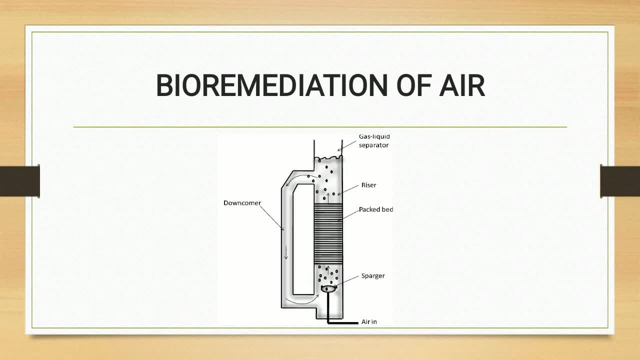 Also, there are chances that the products of degradation can be toxic. In most cases they are not toxic, So it is possible that from the organism is converting one toxic product into another toxic product. That is also possible. Also, these are organisms. 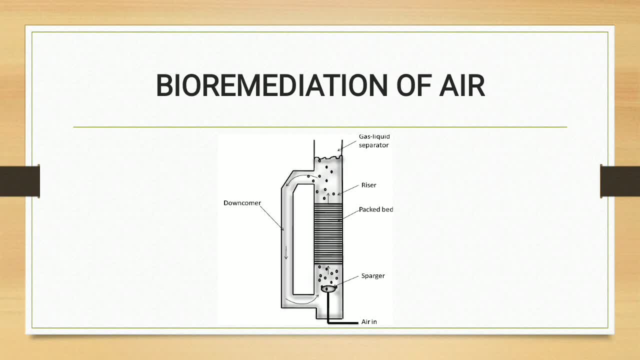 So they are very specific and the bioremediation is based on a lot of factors. Temperature, pH, and the entire environment is going to decide whether bioremediation is going to happen well or not. Also, the time taken is very long.